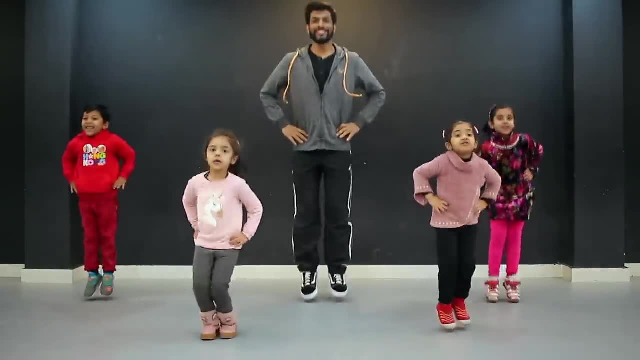 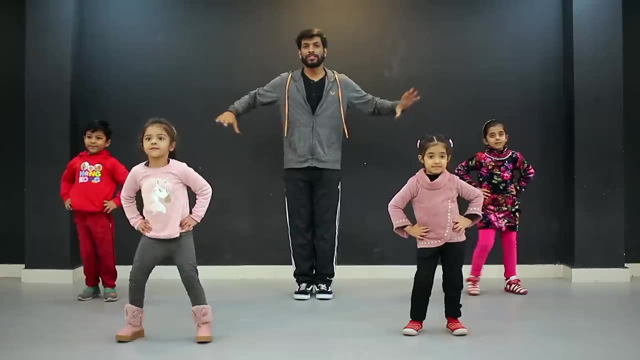 One more, One second, Five, six, seven. start One, two, three, four, five, six, seven, eight. Now we will start with this. Second: Hands on your waist, Open your legs Easy, Let's go. 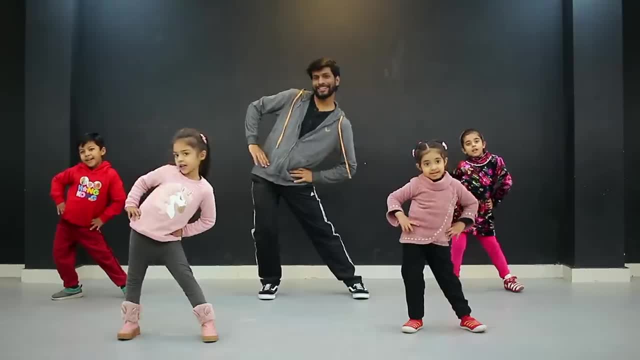 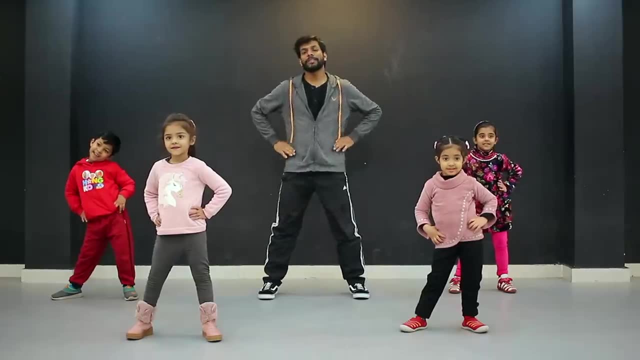 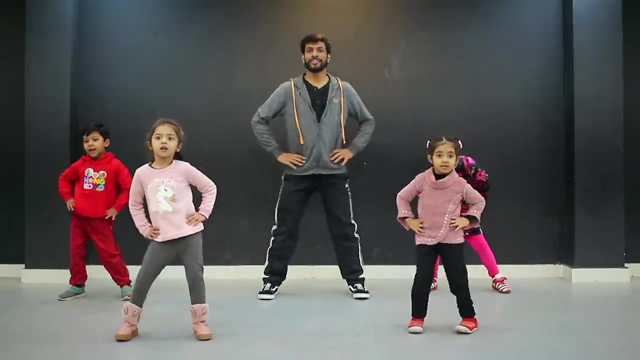 Let's go Right, left, right, left, right, left, Right. Okay, Now tell me, How many counts will you do? Eight, Wow, So I know. Five, six, seven. start One, two, three, four, five, six, seven, eight. 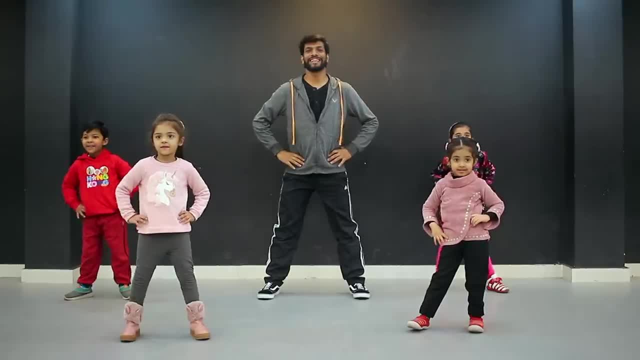 Chee-dee, my little chee-dee. One, second, Five, six, seven go One, two, three, four, five, six, seven, eight. Chee-dee, my little chee-dee. 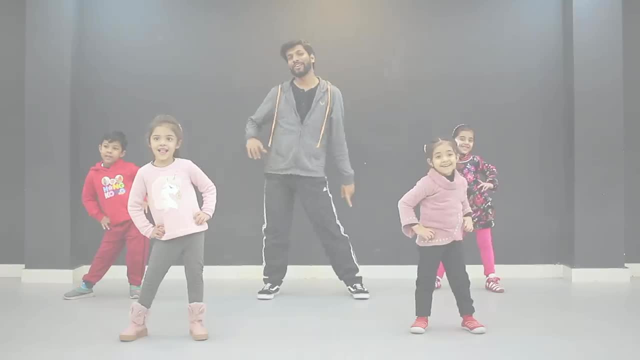 One, two, three, four, five, six, seven, eight, Chee-dee, Chee-dee, Chee-dee. Good, Okay, Now let's move on to the third step. What is the third step? 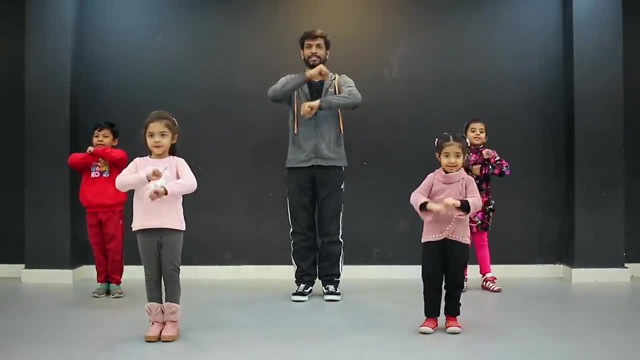 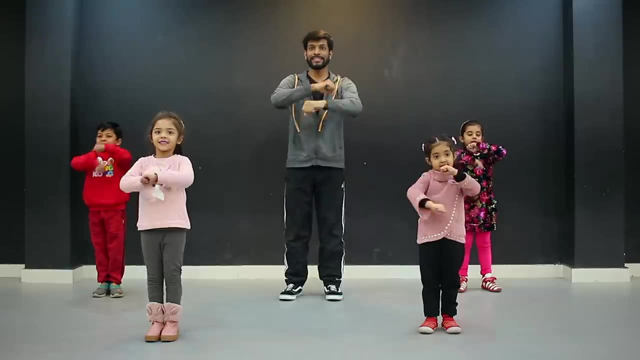 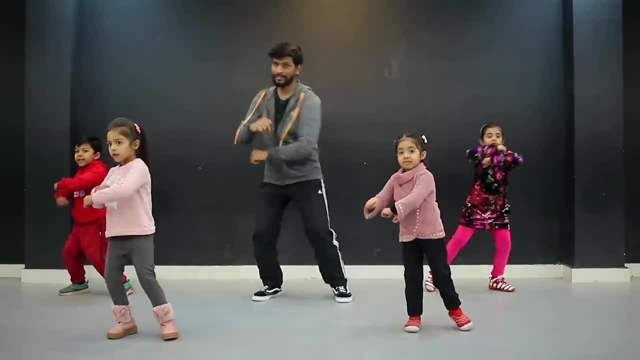 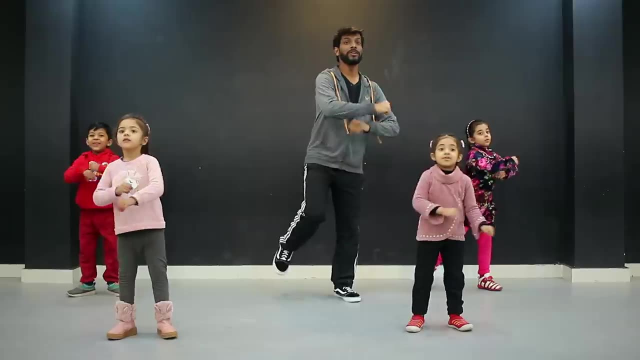 Left side: Four, five, six, seven, eight. Right side, Left side, Very slow: One, two, Roll your hand, Roll your hands a little. Do your hands like this: One, two, Three, Four, five, six, seven, eight. 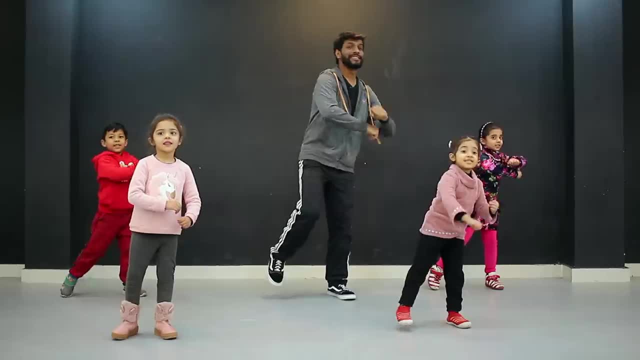 Ch боль. Roll your hands. Roll your hands. Roll your hands One, two, Four, five, six, seven, eight. What happened? I didn't roll my hands. Get back to your position, Roll your hands like this: 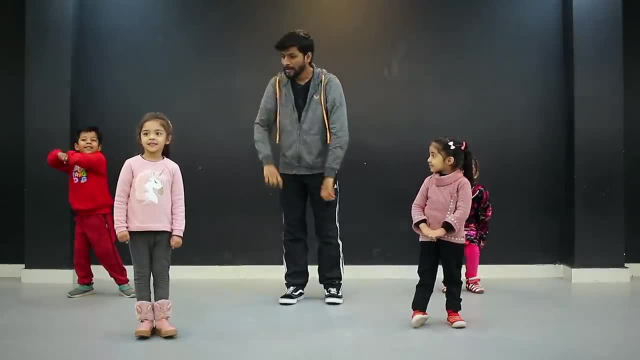 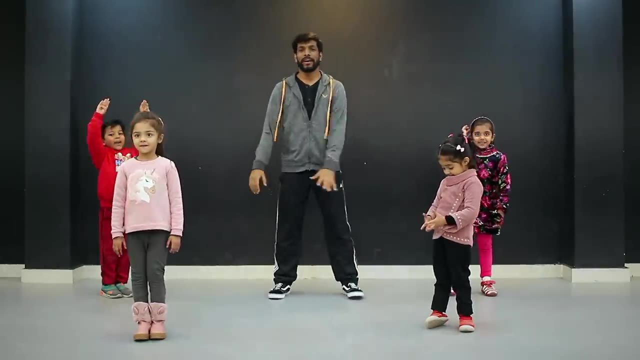 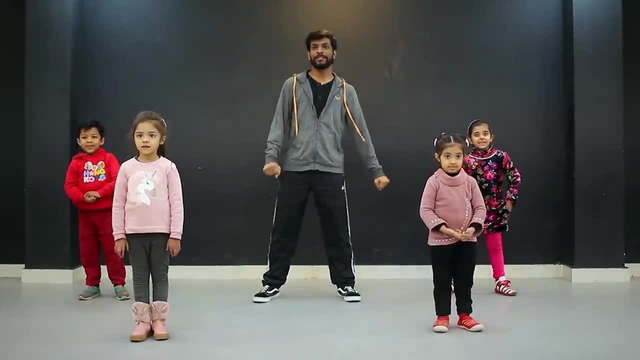 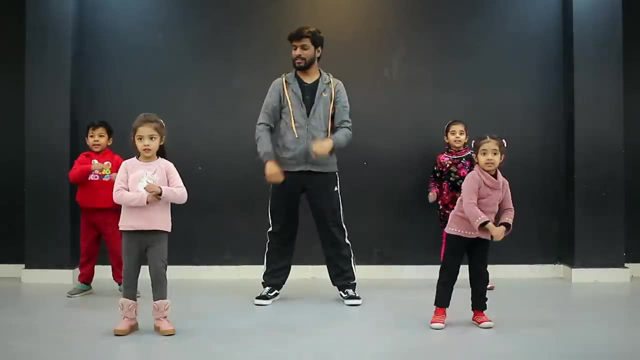 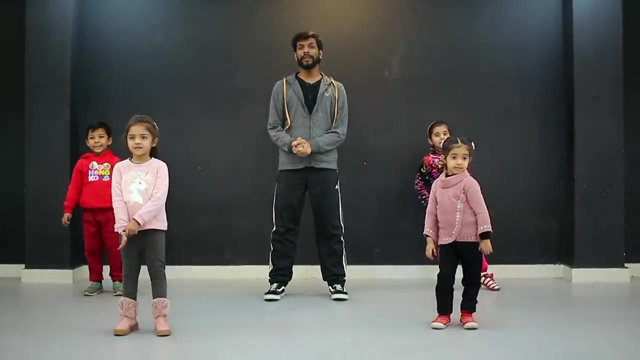 Let's do it again. Let's do five, six, seven. go One, two, three, four, five, six, seven, eight. How are you doing? Okay, so now we will move to the fourth step. Which step is this? 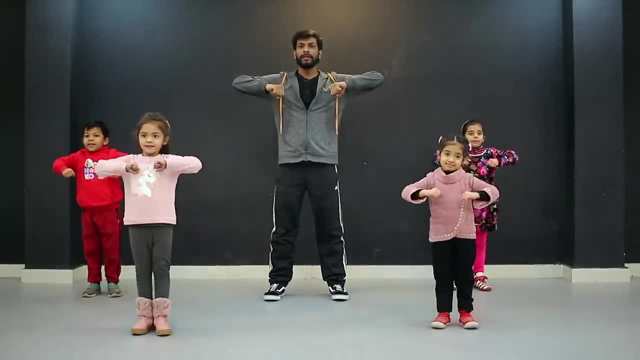 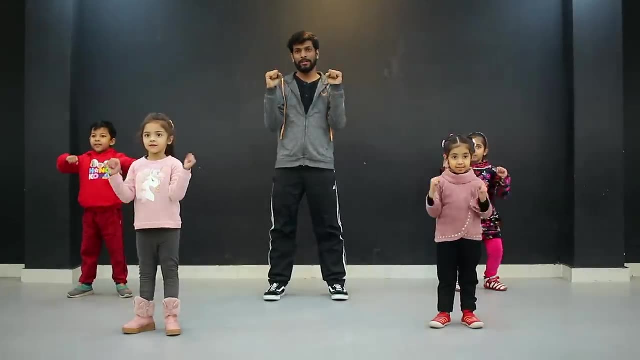 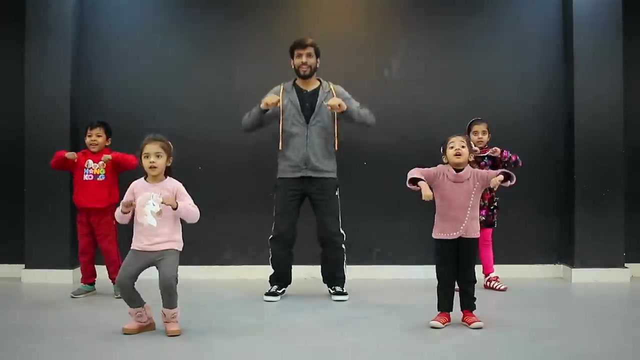 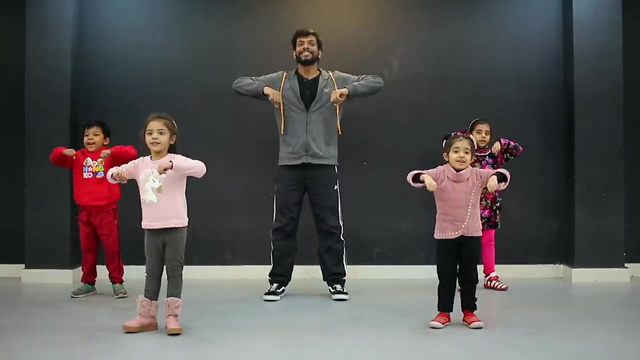 Both, Both hands here, Knees down, knees straight, Knees down, knees straight. Easy, Now we will do handshake: Hands down, hands straight Down up. Let's connect Five, six, seven. go One, two, three, four, five, six, seven, eight. 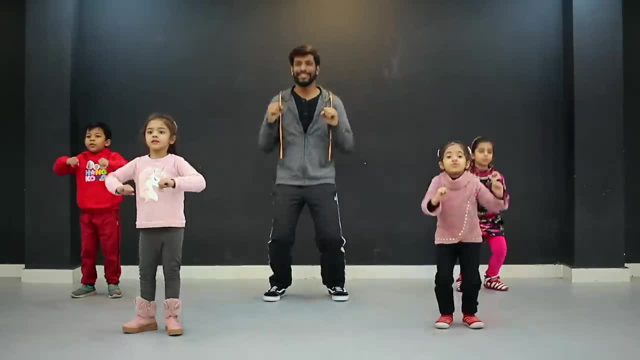 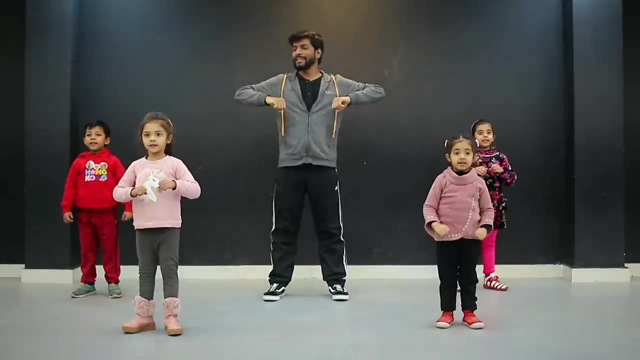 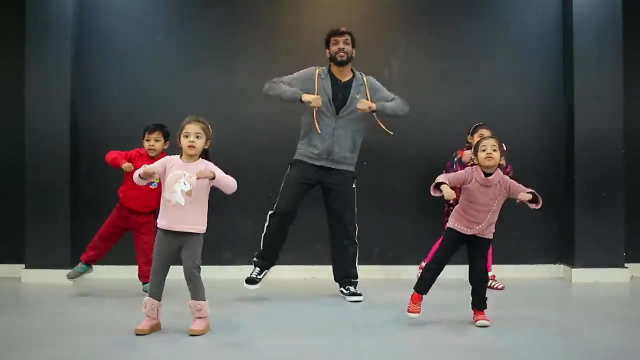 Nice: One, second, One, two, three, four, five, six, seven, eight Nice. Now move to the right and left. One, let us say five, six, seven go. One, two, three, four, five, six, seven, eight. 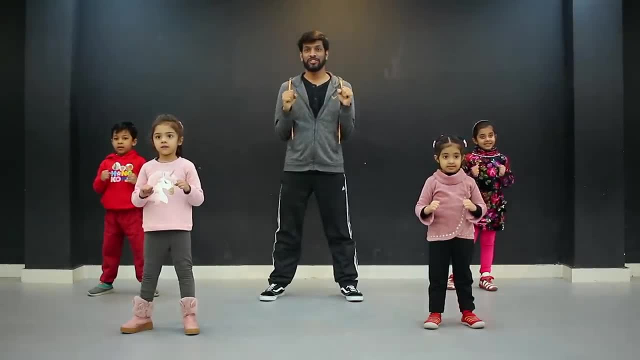 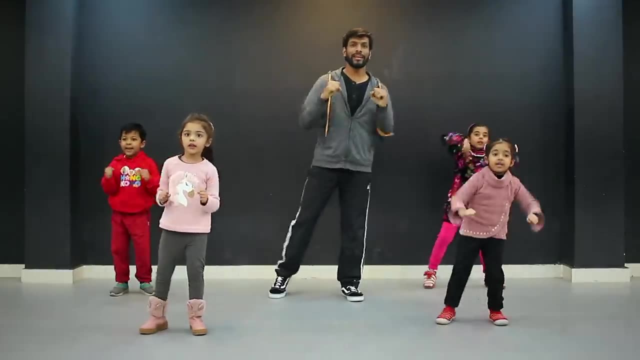 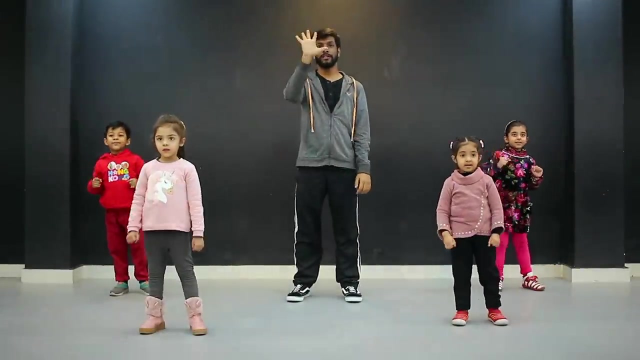 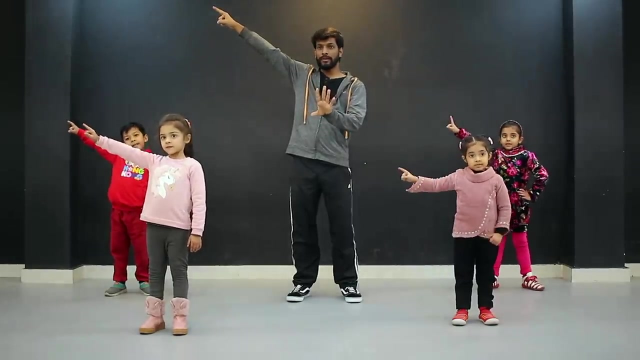 Knees down. 엗. One, two, three, four, five, six, seven, eight. Isabelle, how you doing Very good. Okay, let us move to our fifth step: Five, six, seven go. Now we are going to turn the goal, but we are going to do it slowly, okay. 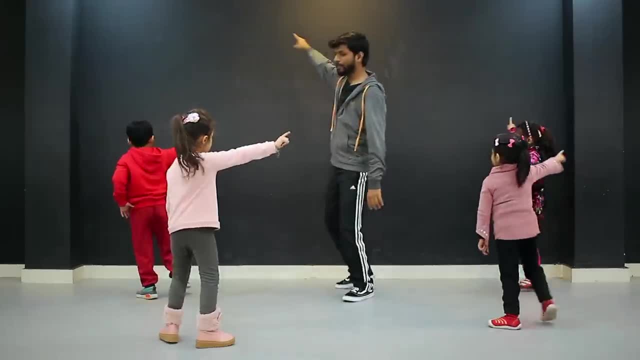 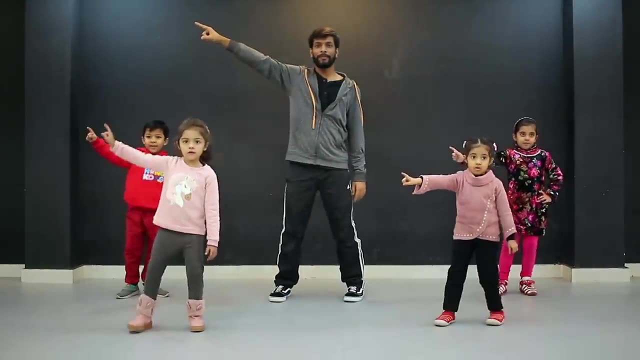 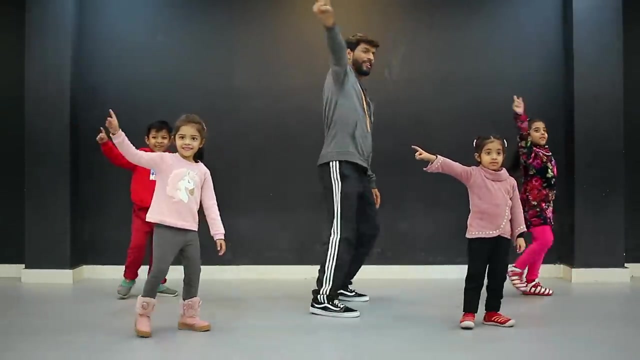 Step, step, step, step Once again. step 2,, 3, stop Once again. 1,, 2,, 3, stop Once again. 1,, 2,, 3, stop. Now we are going to count to 8,, 5,, 6,, 7,, 8.. 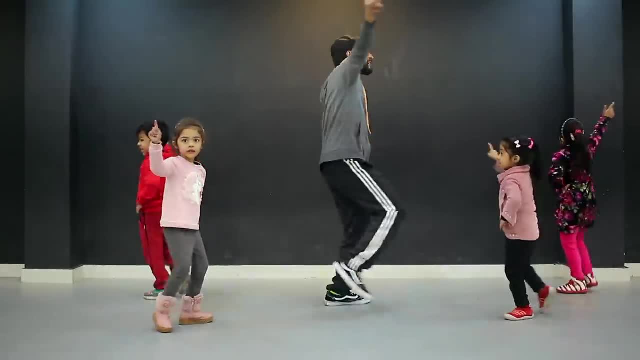 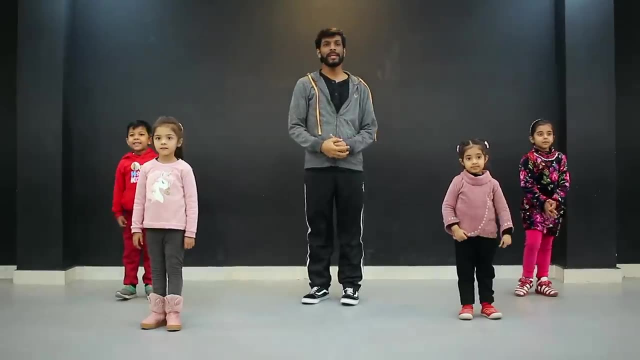 1,, 2,, 3,, 4,, 5,, 6,, 7, 8.. Very good, Okay, did you understand? Yes, What is this step called Surgeon? What Surgeon Surgeon? 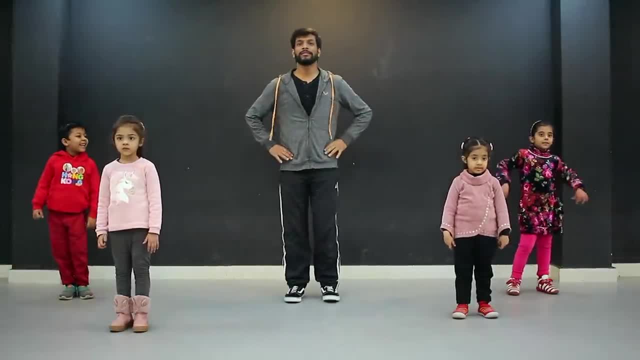 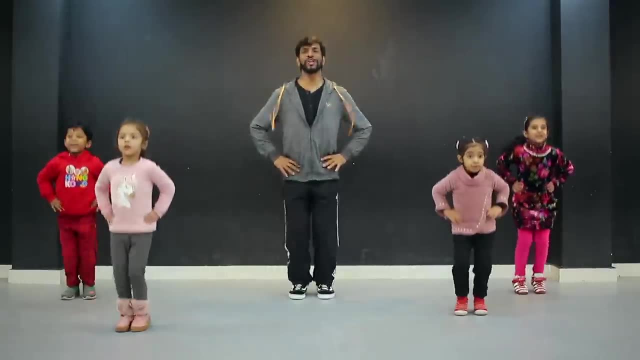